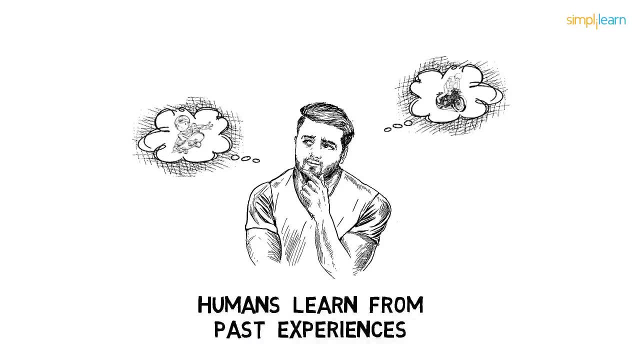 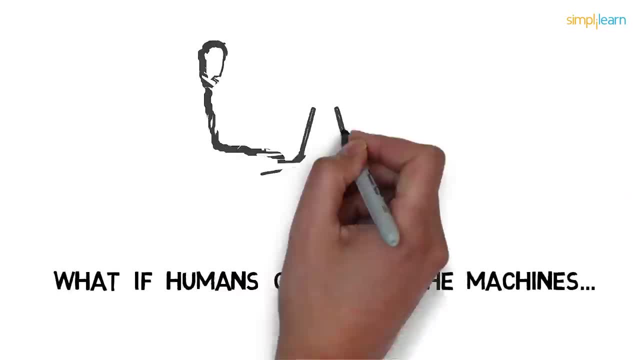 We know humans learn from their past experiences and machines follow instructions given by humans. but what if humans can train the machines to learn from their past data and do what humans can do, and much faster? well, that's called machine learning, but it's a lot more than just learning. 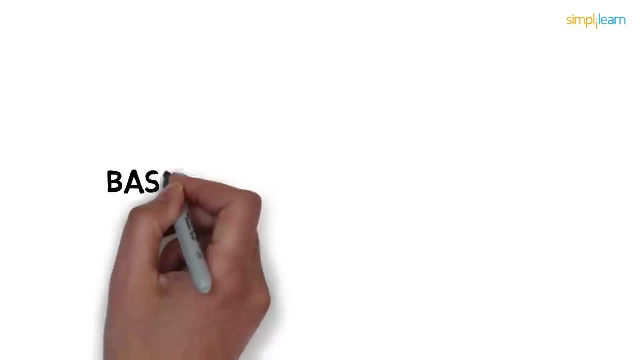 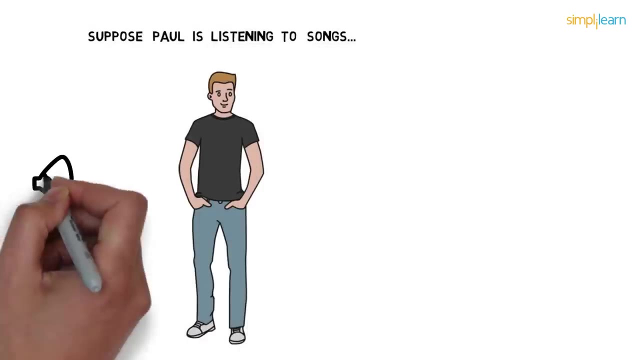 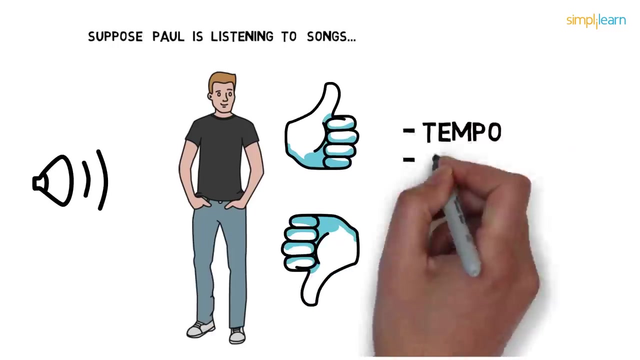 it's also about understanding and reasoning. so today we will learn about the basics of machine learning. so that's paul. he loves listening to new songs. he either likes them or dislikes them. paul decides this on the basis of the song's tempo, genre, intensity and the gender of 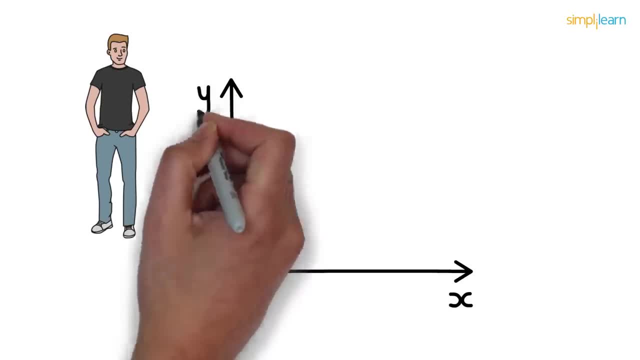 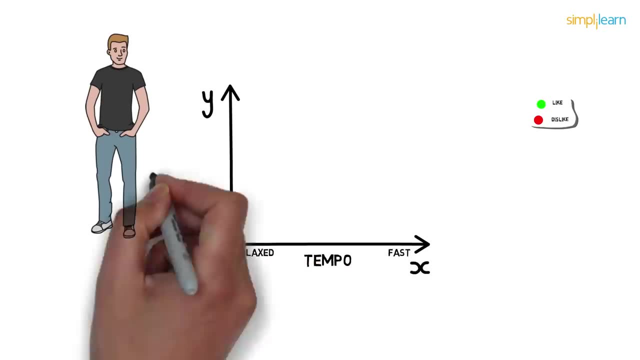 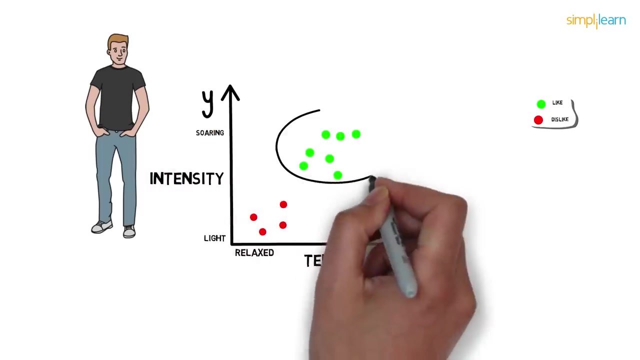 voice for simplicity, let's just use tempo and intensity for now. so here, tempo is on the x-axis, ranging from relaxed to fast, whereas intensity is on the y-axis, ranging from light to soaring. we see that paul likes the song with fast tempo and soaring intensity, while he dislikes the song. 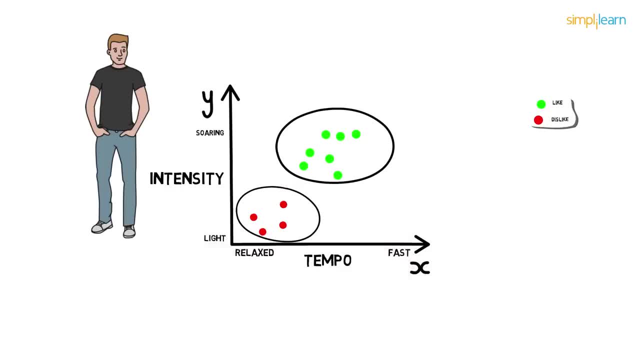 with relaxed tempo and light intensity. so now we know paul's choices. let's say paul listens to a new song. let's name it as song a song a has fast tempo and a soaring intensity, so it lies somewhere here. looking at the data, can you guess whether paul will like the song or not. correct so paul. 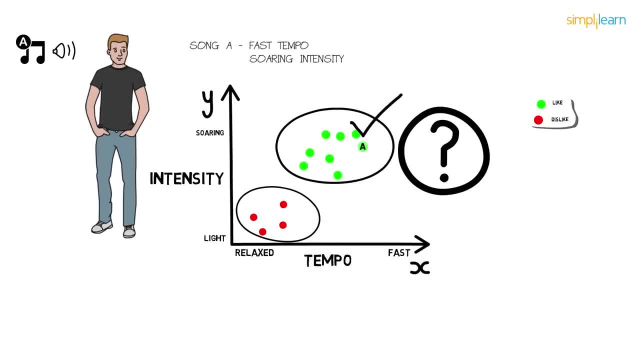 likes this song. by looking at paul's past choices, we were able to classify the unknown song very easily, right? let's say now paul listens to a new song, let's label it as song b. so song b lies somewhere here, with medium tempo and medium intensity, neither relaxed nor fast, neither light nor soaring. now can you guess whether paul likes? 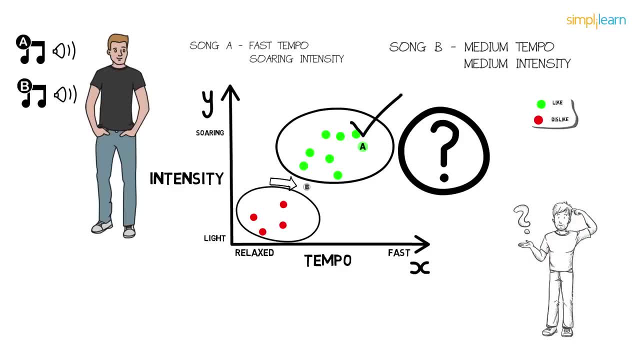 it or not, not able to guess whether paul will like it or dislike it? are the choices unclear, correct? we could easily classify song a, but when the choice became complicated, as in the case of song b, yes, and that's where machine learning comes in. let's see how, in the same example for song b, if we draw a circle around the song b, 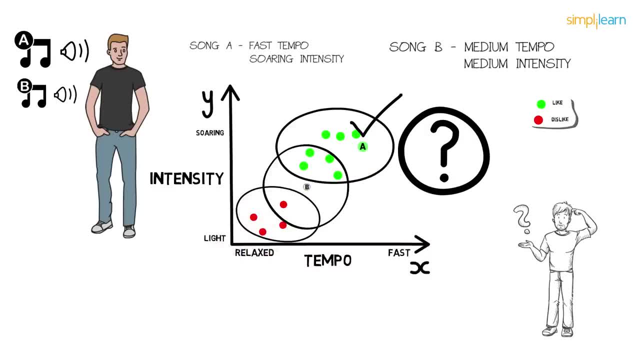 we see that there are four votes for like whereas one vote for dislike. if we go for the majority votes, we can say that paul will definitely like the song. that's all. this was a basic machine learning algorithm. also, it's called k nearest neighbors, so this is just a small example in one. 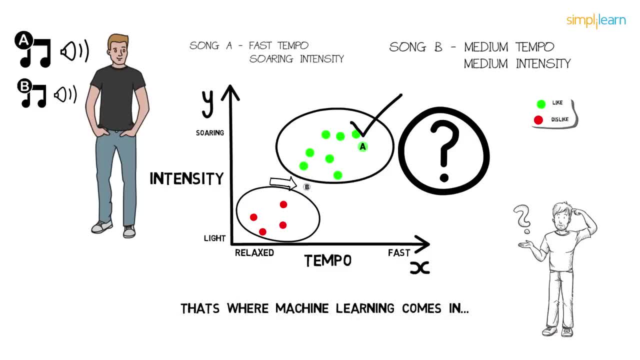 comes in. let's see how. in the same example for song b, if we draw a circle around the song b, we see that there are four votes for like, whereas one vote for dislike. if we go for the majority votes, we can say that paul will definitely like the song. that's all. this was a basic machine learning. 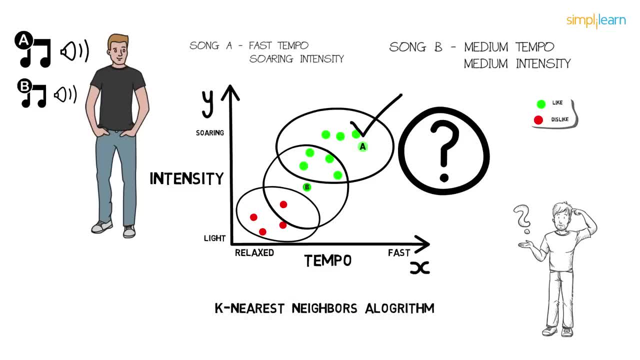 algorithm. also, it's called k- nearest neighbors. so this is just a small example in one of the many systems. quite easy, right? believe me it is. but what happens when the choices become complicated, as in the case of song b? that's when machine learning comes in. it learns the data, builds the prediction. 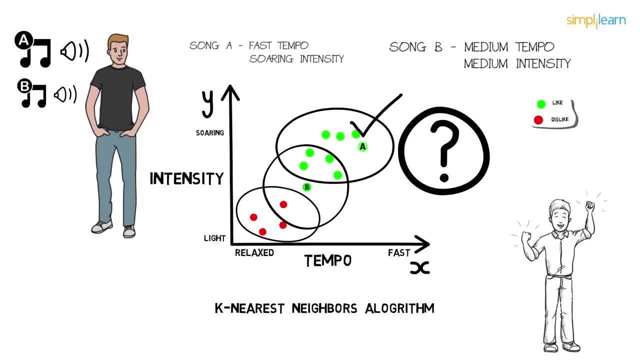 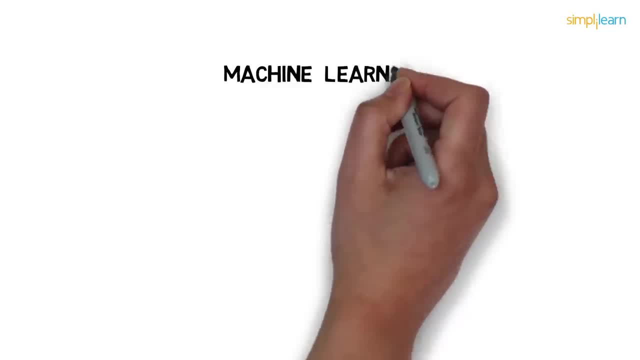 model and when the new data point comes in, it can easily predict for it. more the data, better the model, higher will be the accuracy. there are many ways in which the machine learns. it could be either supervised learning, unsupervised learning or reinforcement learning. let's first quickly. 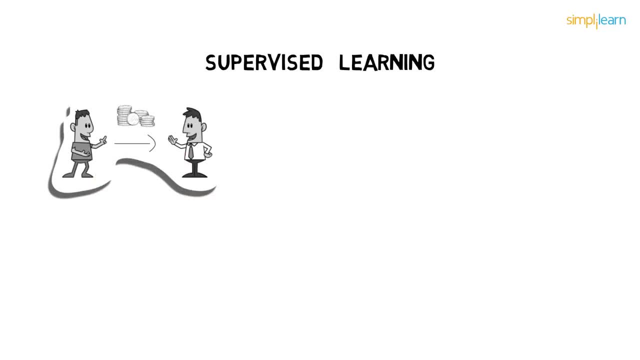 talk about supervised learning. suppose your friend gives you one million coins of three different currencies, say one rupee, one euro and one dirham. each coin has different weights. for example, a coin of one rupee weighs three grams, one euro weighs seven grams and one dirham weighs four grams. your 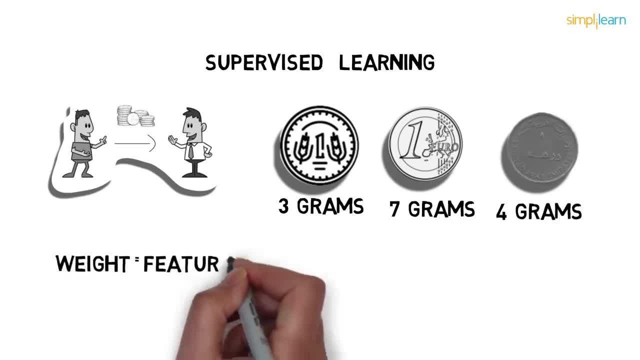 model will predict the currency of the coin. here, your weight becomes the feature of coins, while currency becomes their label. when you feed this data to the machine learning model, it learns which is associated with which label. for example, it will learn that if a coin is of three grams, it will be. 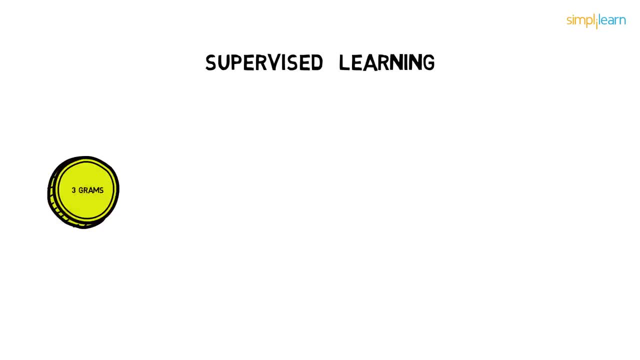 a one rupee coin. let's give a new coin to the machine. on the basis of the weight of the new coin, your model will predict the currency. hence supervised learning uses labeled data to train the model. here, the machine knew the features of the object and also the labels associated with. 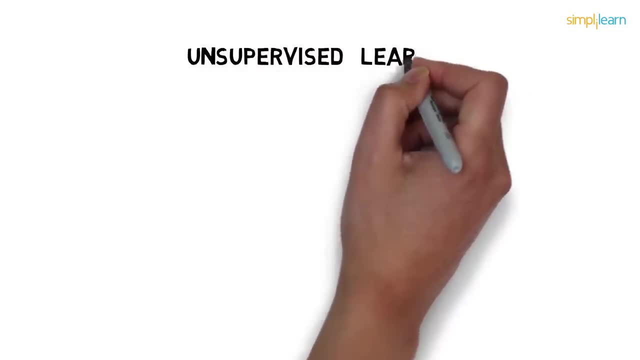 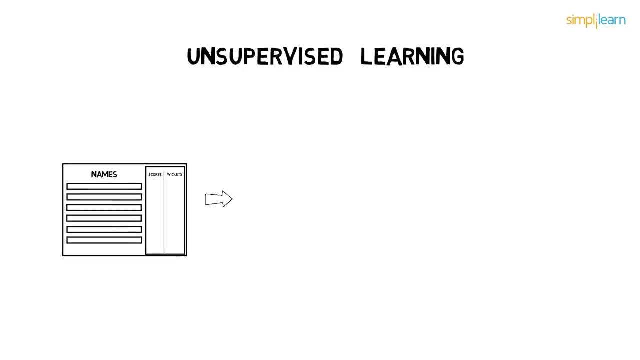 those features. on this note, let's move to unsupervised learning and see the difference. suppose you have cricket data set of various players with their respective scores and wickets taken. when we feed this data set to the machine, the machine identifies the pattern of player performance, so it plots this data with the respective wickets on the x-axis. 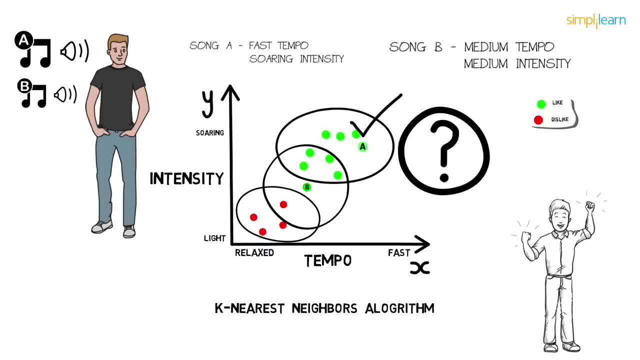 of the many machine learning algorithms. quite easy, right, believe me it is. but what happens when the choices become complicated, as in the case of song b? that's when machine learning comes in. it learns the data, builds the prediction model, and when the new data point comes in, it can easily predict for. 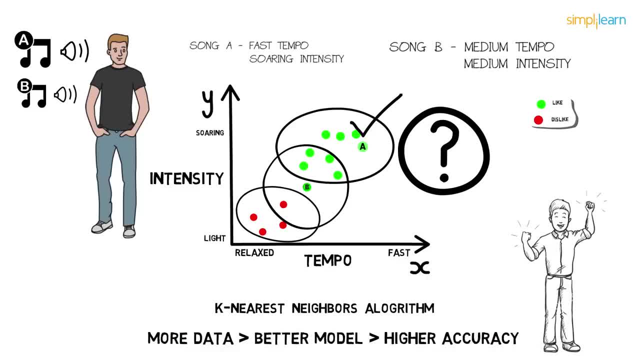 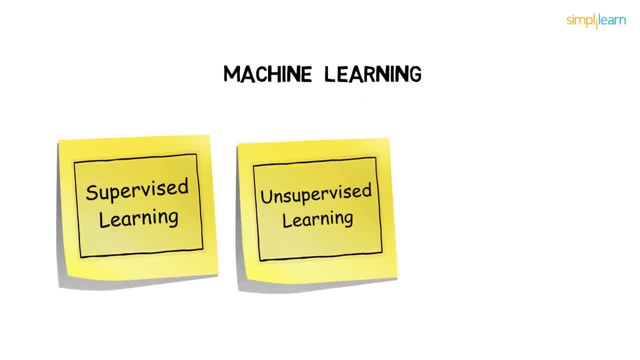 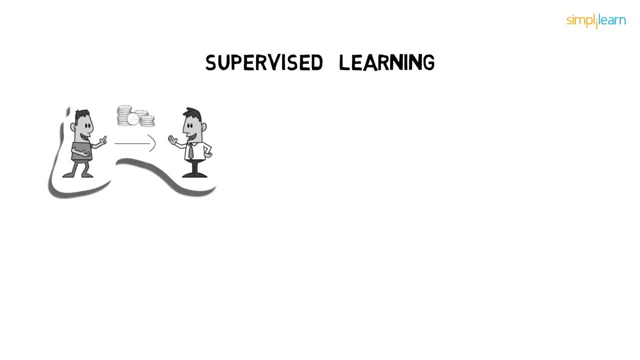 it. more the data, better the model, higher will be the accuracy. there are many ways in which the machine learns. it could be either supervised learning, unsupervised learning or reinforcement learning. it could be supervised learning, unsupervised learning or reinforcement learning. let's first quickly understand supervised learning. suppose your friend gives you one million coins. 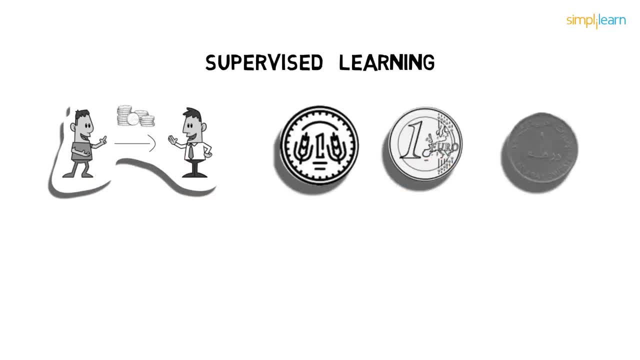 of three different currencies, say one rupee, one euro and one dirham. each coin has different weights. for example, a coin of one rupee weighs three grams, one euro weighs seven grams and one dirham weighs four grams. your model will predict the currency of the coin. here your weight becomes the feature of. 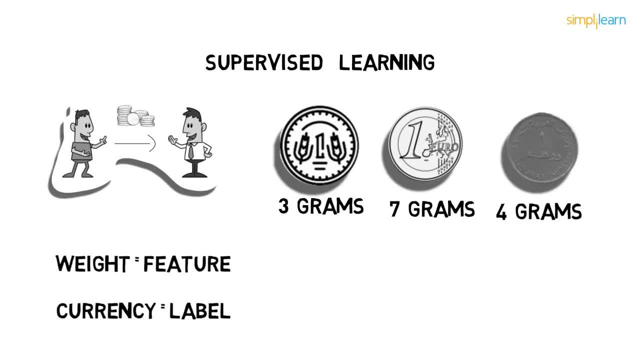 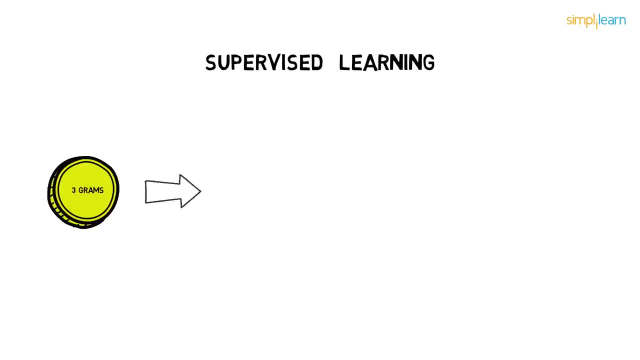 coins, while currency becomes their label. when you feed this data to the machine learning model, it learns which feature is associated with which label. for example, it will learn that if a coin is of three grams, it will be a one rupee coin. let's give a new coin to the machine on the basis of the weight of. 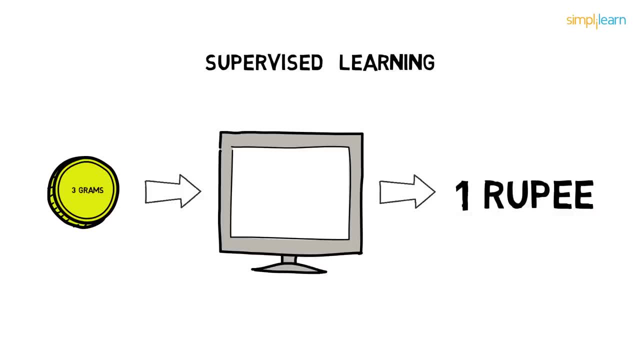 the new coin, your model will predict the currency. hence supervised learning uses labeled data to train the model. here, the machine knew the features of the object and also the labels associated with those features. on this note, let's move to unsupervised learning and see the difference. 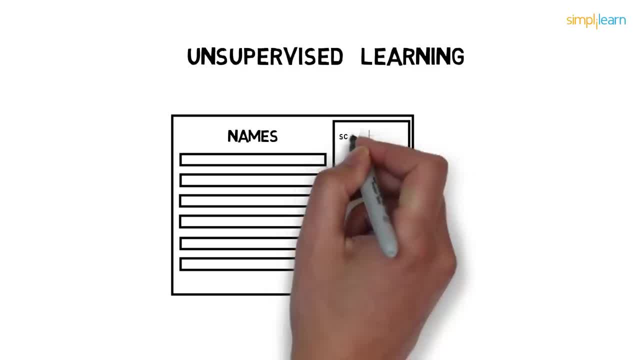 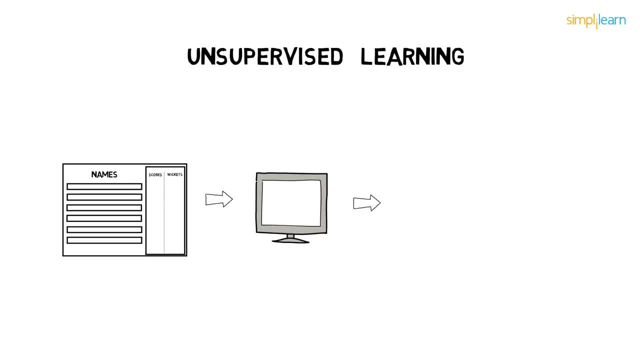 suppose you have cricket data set of various players with their respective scores and the wickets taken. when we feed this data set to the machine, the machine identifies the pattern of player performance, so it plots this data with the respective wickets on the x axis while runs on the y-axis. 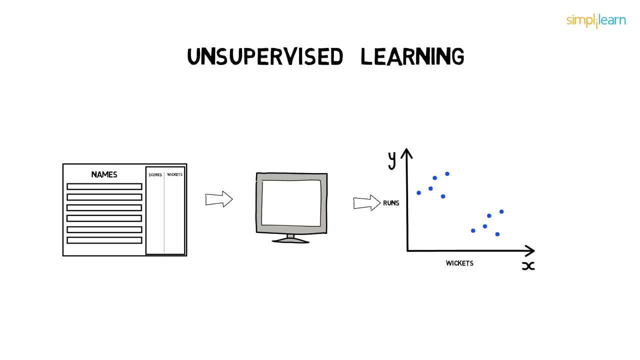 by looking at the data, you'll clearly see that there are two clusters. the one cluster are the players who scored high runs and took less wickets, while the other cluster is of the players who scored less runs but took many wickets. so here we interpret these two. 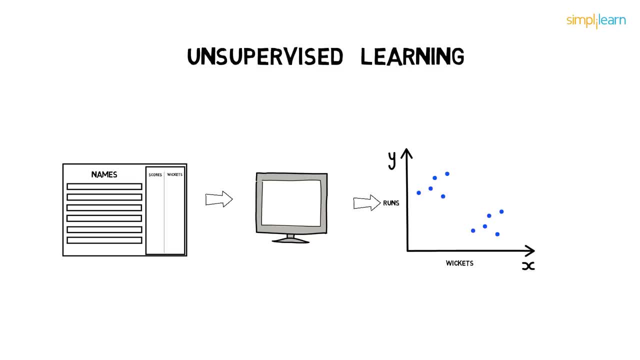 while runs on the y-axis. while looking at the data, you'll clearly see that there are two clusters. the one cluster are the players who scored high runs and took less wickets, while the other cluster is of the players who scored less runs but took many wickets. so here we interpret these two clusters as: 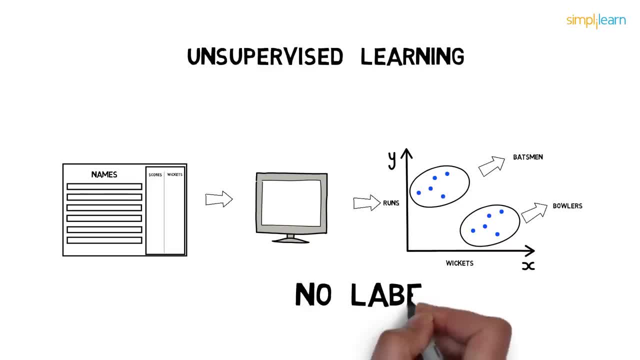 an important point to note here is that there were no labels of batsmen and bowlers, hence the learning with unlabeled data is unsupervised learning. so we saw supervised learning where the data was labeled and the unsupervised learning where the data was unlabeled. 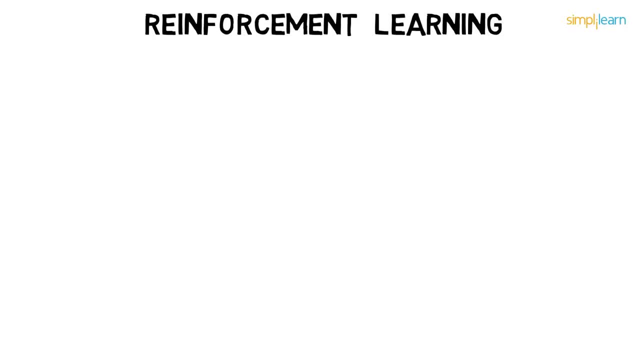 and then there is reinforcement learning, which is reward based learning, or we can say that it works on the principle of feedback here. let's say you provide the system with an image of a dog and ask it to identify it. the system identifies it as a cat, so you give a negative feedback. 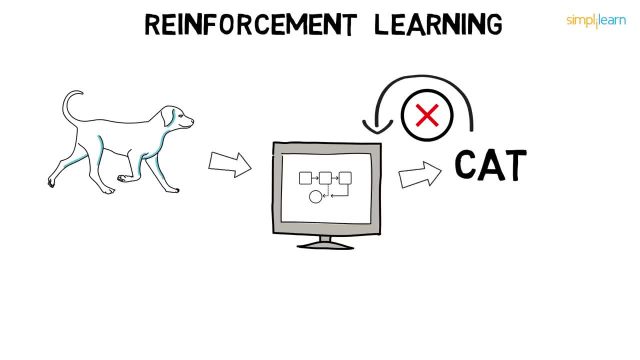 to the machine saying that it's a dog's image. the machine will learn from the feedback and, finally, if it comes across any other image of a dog, it will be able to classify it correctly. that is reinforcement learning, to generalize machine learning model. let's see a flow chart. 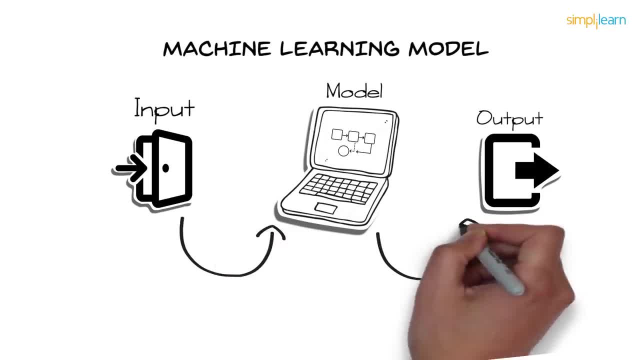 input is given to a machine learning model, which then gives the output according to the algorithm applied. if it's right, we take the output as a final result. else we provide feedback to the training model and ask it to predict until it learns. i hope you've understood. supervised. 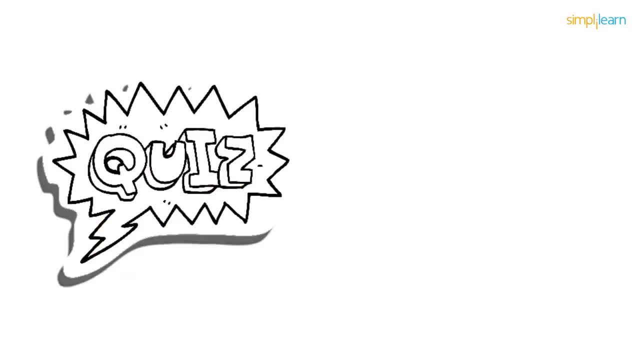 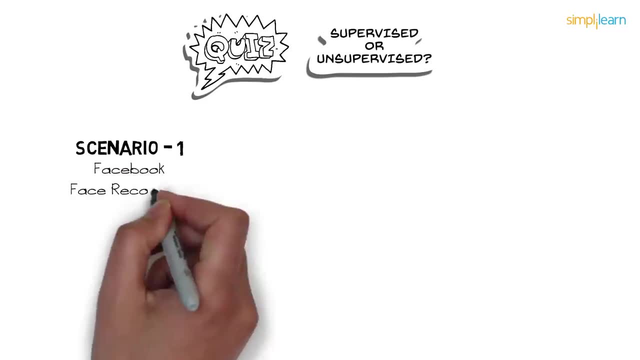 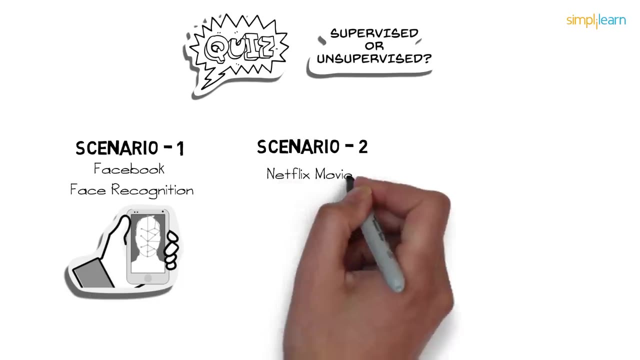 unsupervised learning. so let's have a quick quiz. you have to determine whether the given scenarios uses supervised or unsupervised learning, simple, right. scenario 1: facebook recognizes your friend in a picture from an album of tagged photographs. scenario 2: netflix recommends new movies based. 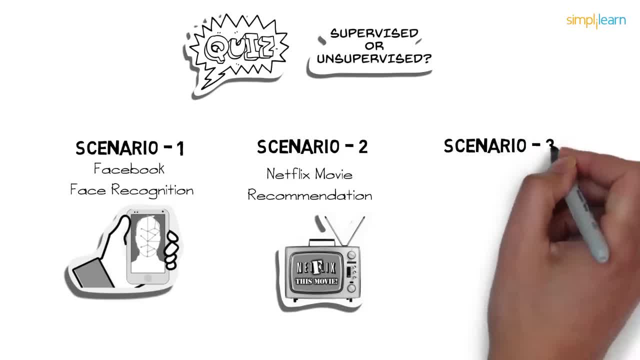 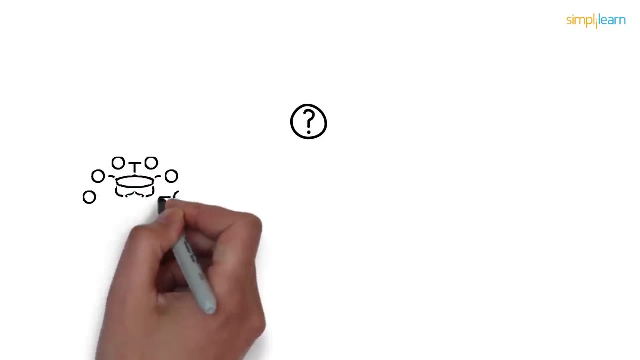 on someone's past movie choices. scenario 3: analyzing bank data for suspicious transactions and flagging the fraud transactions. think wisely and comment below your answers. moving on, don't you sometimes wonder how is machine learning possible in today's era? well, that's because today we have humongous data available. everybody is online, either making 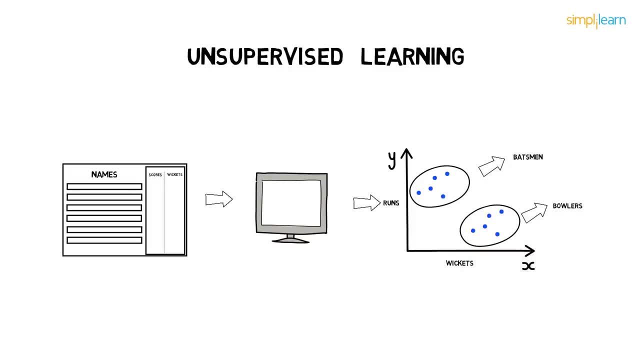 as batsmen and bowlers. An important point to note here is that there were no labels of batsmen and bowlers. Hence the learning with unlabeled data is unsupervised learning. So we saw supervised learning where the data was labeled and the unsupervised learning where the data was unlabeled. 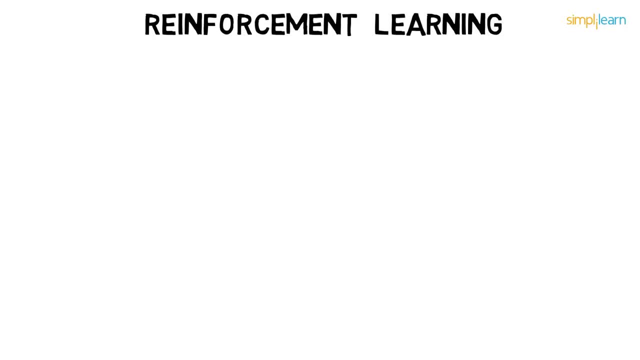 And then there is reinforcement learning, which is reward-based learning, or we can say that it works on the principle of feedback Here, let's say you provide the system with an image of a dog and ask it to identify it. The system identifies it as a cat, So you give a negative feedback to. 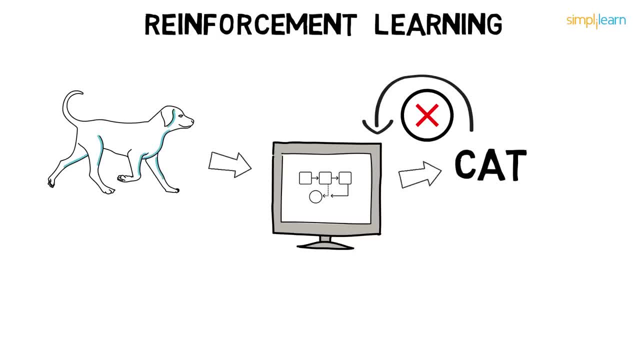 the machine saying that it's a dog's image. The machine will learn from the feedback and finally, if it comes across any other image of a dog, it will be able to classify it correctly. That is reinforcement learning. To generalize machine learning model, let's see a flowchart. Input is: 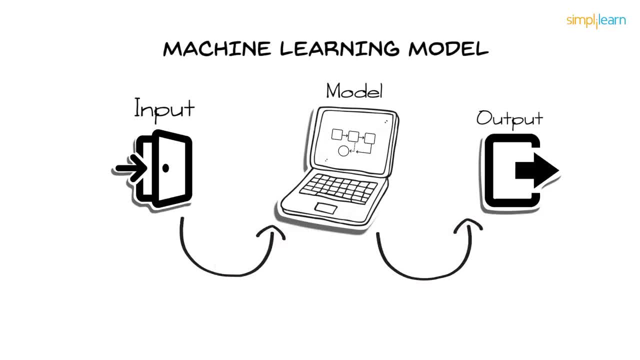 given to a machine learning model, which then gives the output according to the algorithm applied. If it's right, we take the output as our final result. Else, we provide feedback. We give feedback to the training model and ask it to predict until it learns. 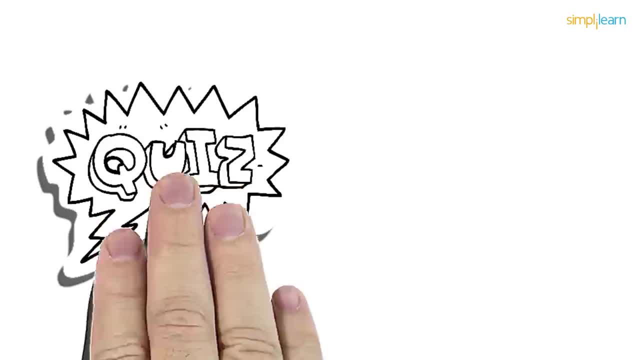 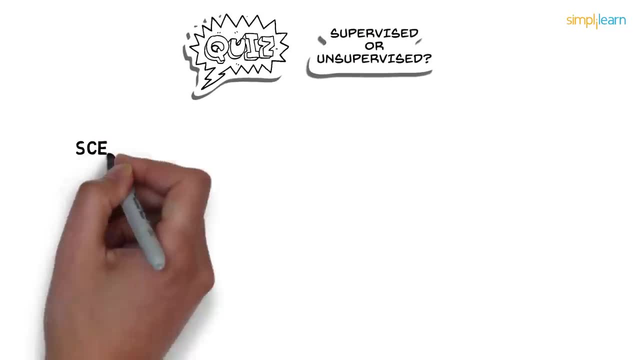 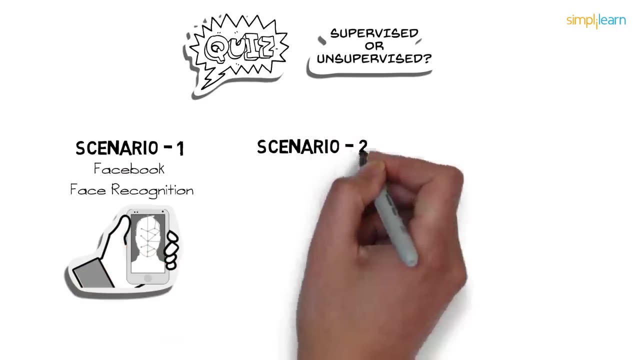 I hope you've understood supervised and unsupervised learning. So let's have a quick quiz. You have to determine whether the given scenario uses supervised or unsupervised learning. Simple right Scenario 1. Facebook recognizes your friend in a picture from an album of tagged photographs. 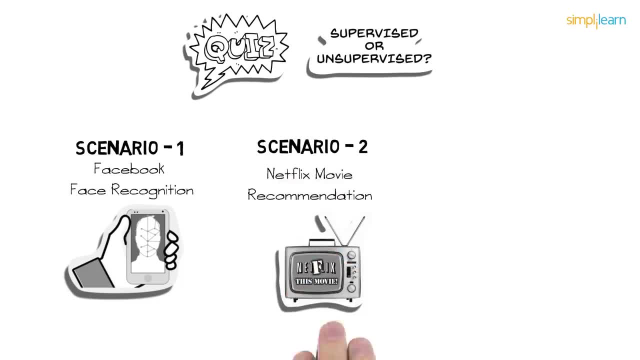 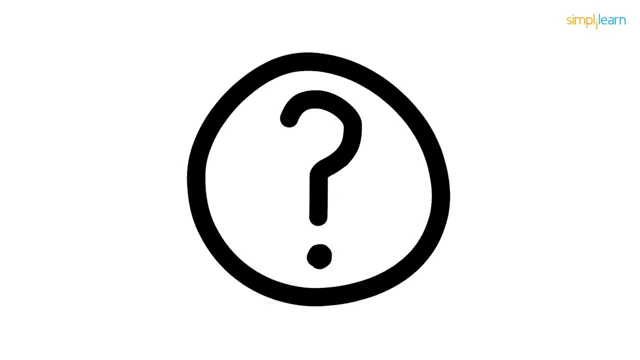 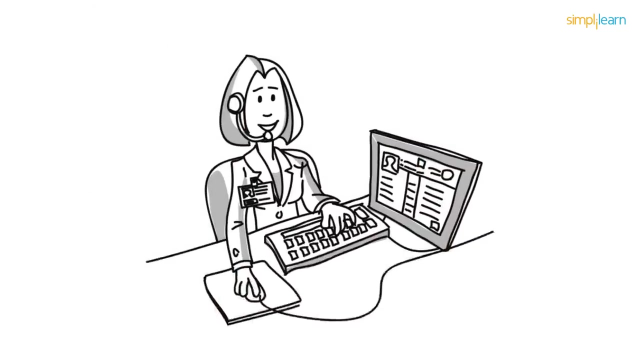 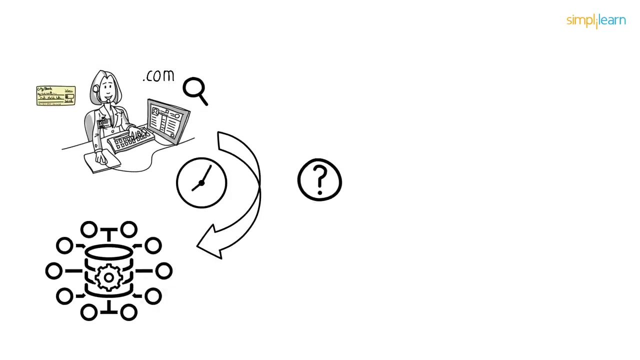 Scenario 2. Netflix recommends new movies based on someone's past movie choices. Scenario 3. Netflix promises to date your friend's past and how she will react to it. So that's screaming smart and willing. Next is the second scenario. 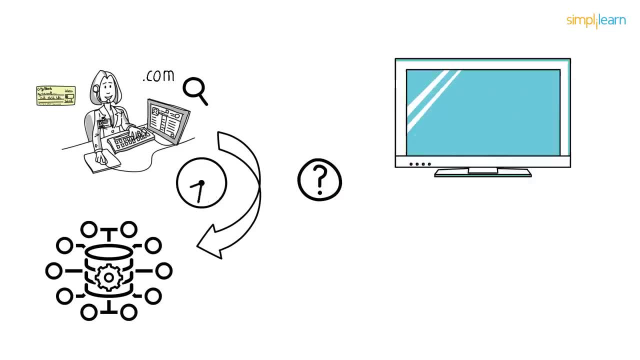 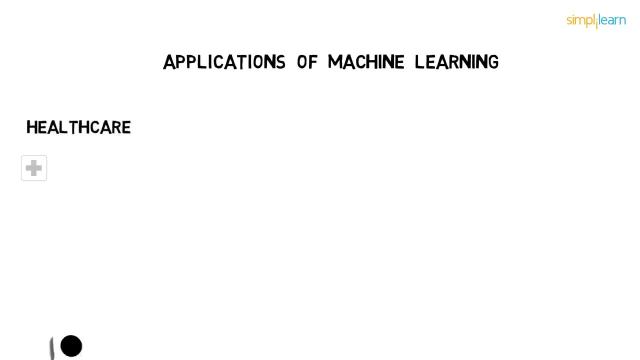 Scenario 4. of computers have largely increased, which helps them to process such a huge amount of data at hand without any delay. And yes, computers now have great computational powers. So there are a lot of applications of machine learning out there. To name a few, machine learning is used in healthcare, where diagnostics are predicted.